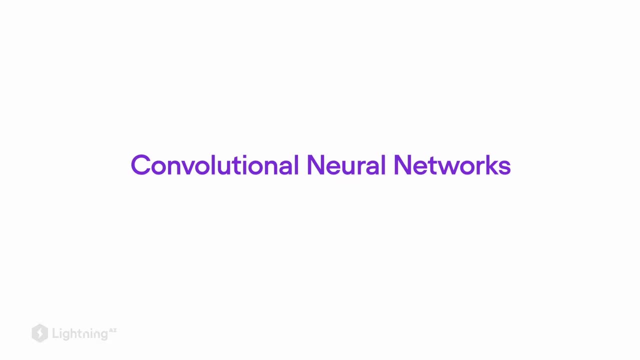 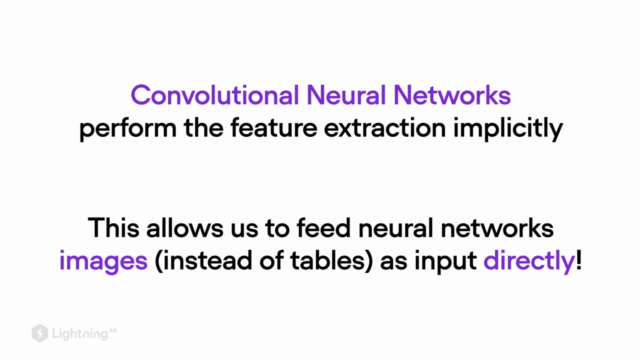 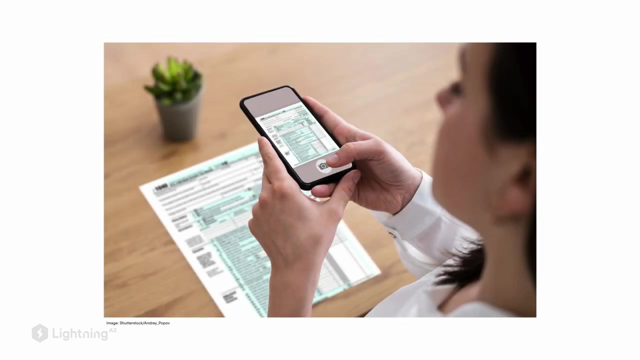 don't have to worry about manual feature extraction. Modern deep learning So this allows us to feed the neural networks image data as input directly, so we can skip the manual feature extraction step. So popular examples of convolutional networks are optical character recognition software that you may have already used on your phone Or, for example, 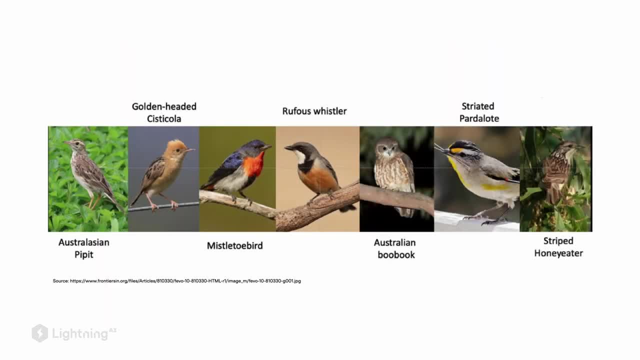 if you are interested in identifying different birds in your garden, you can implement a bird classifier using a convolutional neural network. So this allows us to feed the neural networks image data as input directly, so we can skip the manual feature extraction step. So when we use modern deep learning architectures such as convolutional neural networks. we don't have to worry about manual feature extraction software that you may have already used on your phone Or, for example, if you are interested in identifying different birds in your garden, you can implement a bird classifier using a. 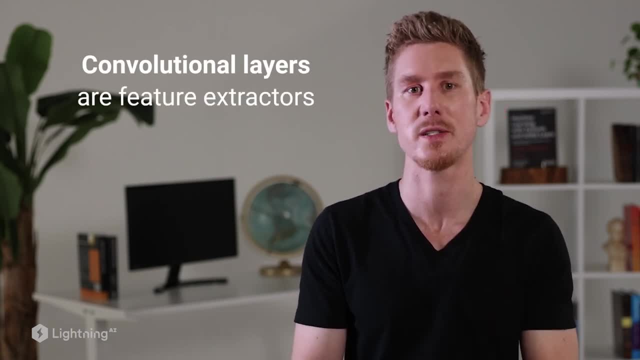 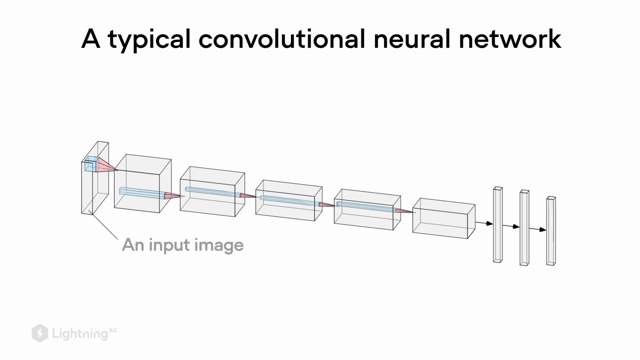 convolutional neural network. So one of the key features of convolutional neural networks are the convolutional layers. The convolutional layers are feature extractors. To make this a little bit more concrete, consider this architecture sketch of a typical convolutional neural network. So here this convolutional network receives an input image. Typically, 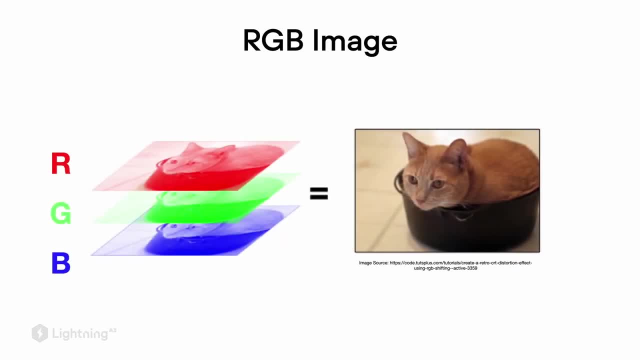 that's an RGB image. RGB stands for red, green and blue, which are the different color channels that make up this image. You can think of an RGB image as a stack of matrixes. So you can think of an RGB image as a stack of matrixes. So you can think of an RGB image as a stack. 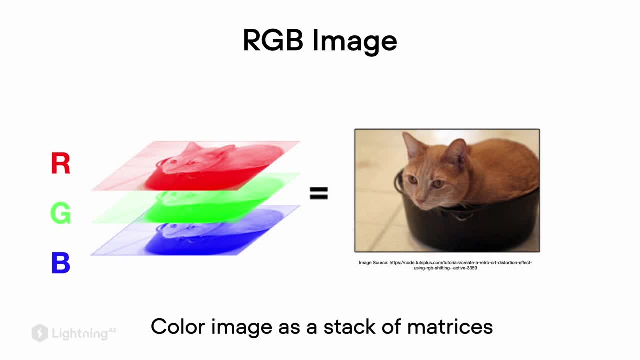 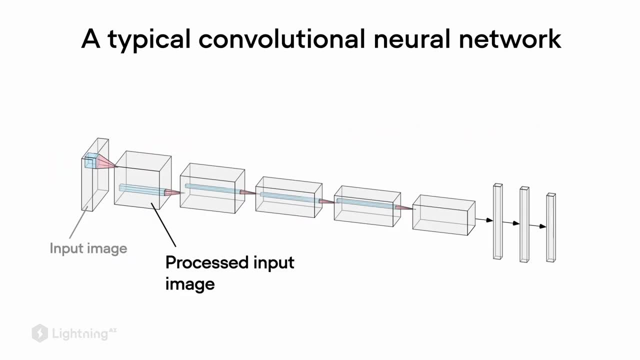 of matrices. So each matrix has a height and a width dimension, And here we have three different matrices stacked together: a red matrix, a green matrix and a blue matrix. So each block here in this figure represents one convolutional layer And the convolutional 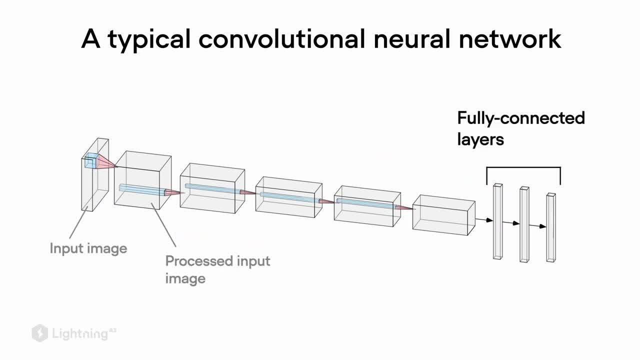 layers- here we have five of them- are then followed by fully connected layers. So in this case we have three fully connected layers, two hidden layers and one output layer, And actually we can think of these fully connected layers as the multi-layer perceptron. So we 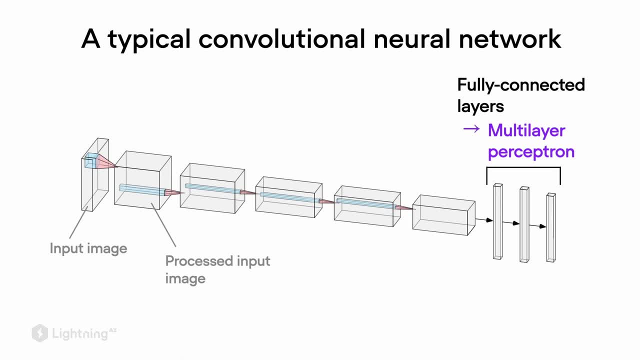 can think of this fully connected layer as the multi-layer perceptron, And actually we can think of these fully connected layers as the multi-layer perceptron. So typically, conventional network architecture consists of a convolutional backbone and this multi-layer perceptron unit, And so, to draw the analogy to the previous units we have at this point, 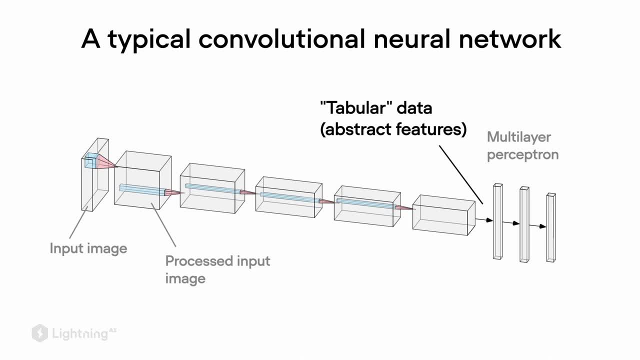 the multi-layer perceptron receives something that kind of represents tabular data. So at this point the multi-layer perceptron part works exactly as before, except this tabular data here was implicitly extracted by the convolutional layers. So in previous units-